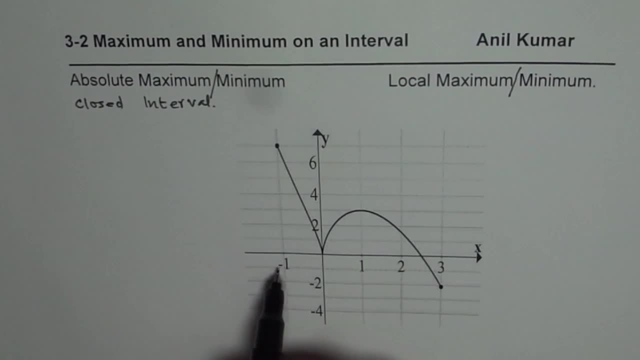 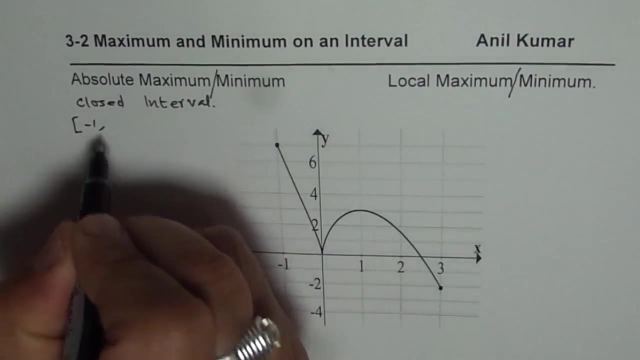 is given in a closed interval. The interval here is from minus one to three. So we'll say: the interval is from minus one to three. right, So in inequalities you could also write this as a closed interval. So we'll say: the interval is from minus one to three. right, So in inequalities. 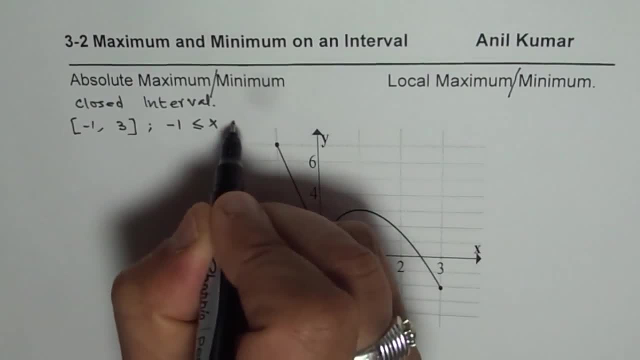 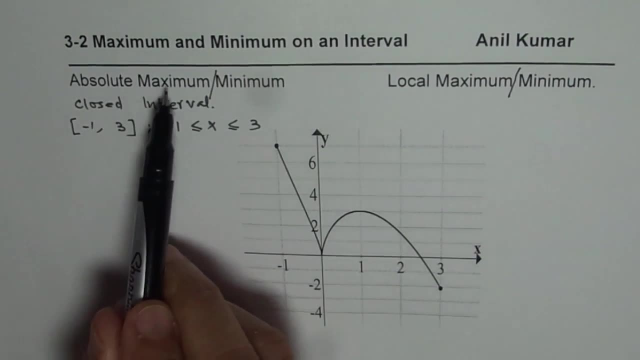 you could also write this as: x is greater than equal to minus one and is less than equal to three. right, That is what? Now let's answer this question: What is the absolute maximum value and what is the absolute minimum value from the given graph in this closed interval, right? So 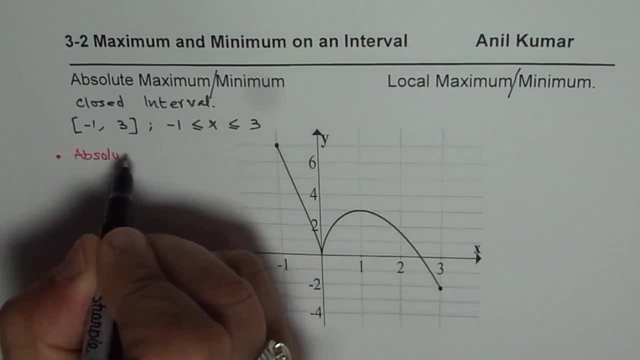 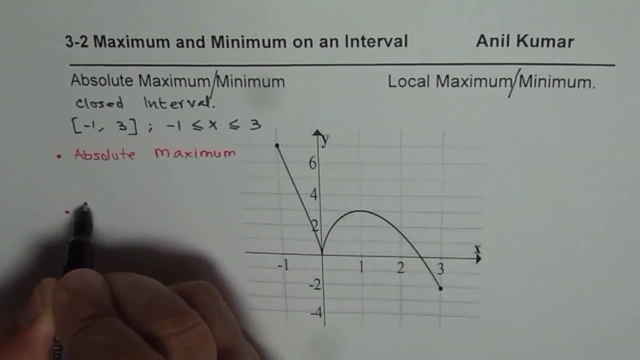 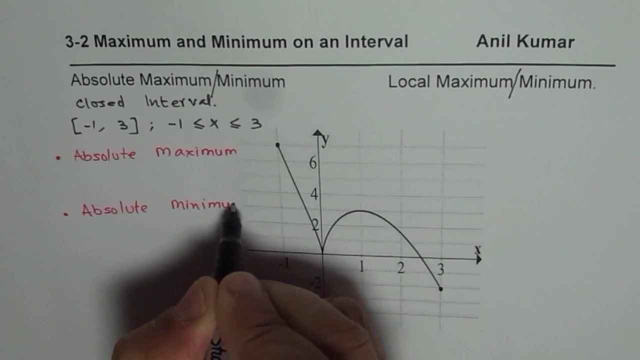 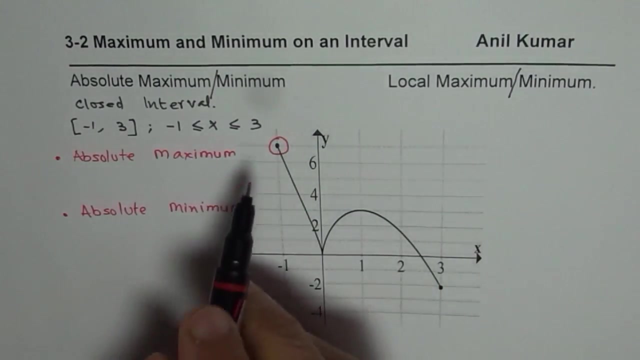 let's find absolute maximum and absolute minimum. So can you tell me what is the absolute maximum value and what is the absolute minimum value from the graph? Well, clearly, in this interval, that point is the absolute maximum highest value in the interval and the minimum. 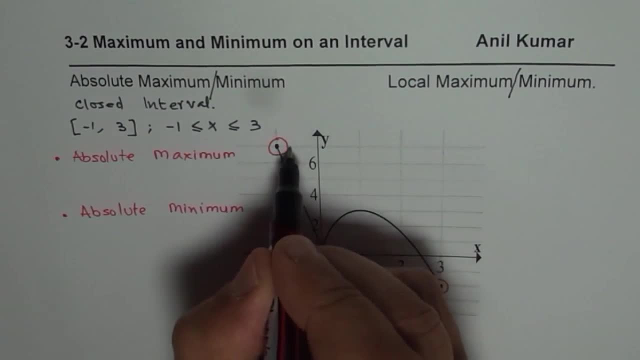 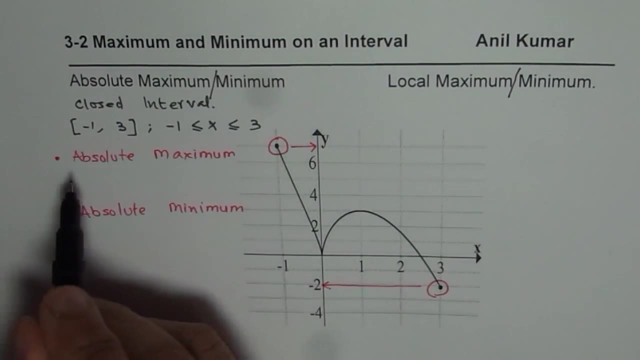 value. is this point right? So we can say: the y values corresponding to these are what we are interested in figuring out, right? So the answer here is that absolute maximum is seven. So this value is seven and absolute minimum is minus two, right, This value of seven? 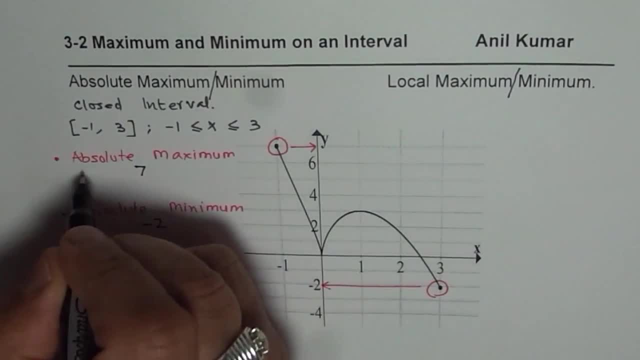 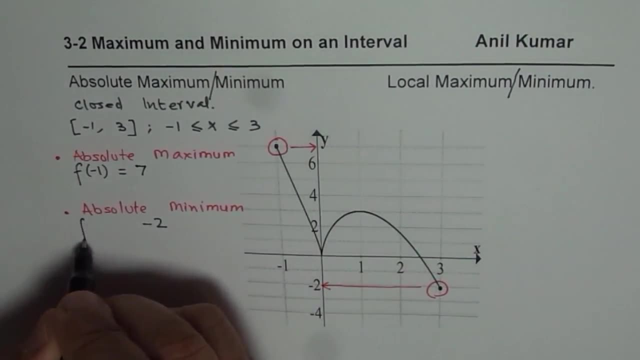 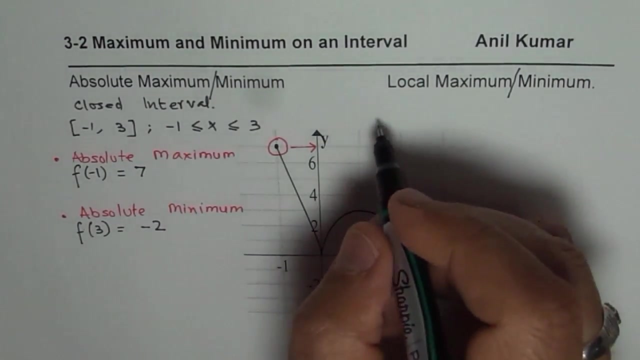 occurs at minus one. So you could write this function as: f of minus one equals to seven is absolute maximum and f of three equals to minus two is absolute minimum. right Now let us look into the other two terms, which are local maximum and local minimum, right? So these two terms which we talk about are local maximum. 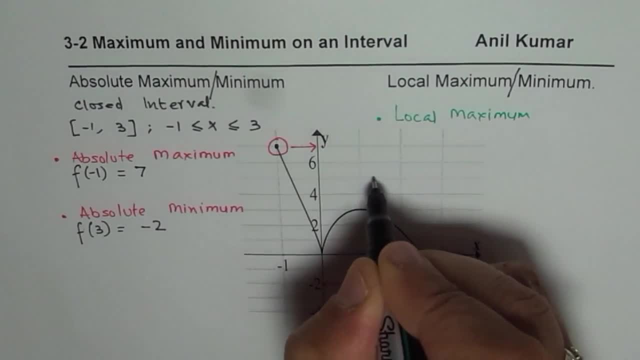 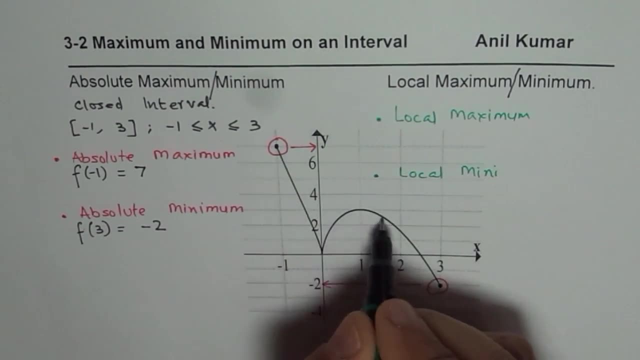 and local minimum right. The difference here is that local means close, in a close vicinity, right. So that is what is a main difference, right? So we look into local. So here you will see that point: within its close vicinity. 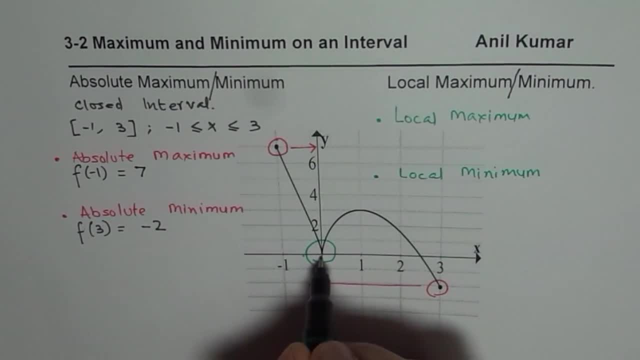 This point is at minimum right And that point is at maximum in its close vicinity. Do you see that part? So those are kind of turning points, cusps or corners. So those values will give you local maximum and minimum values. So answer for us in this case will be: local maximum is at one. 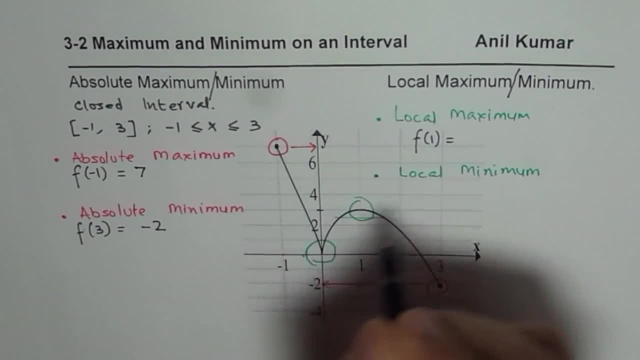 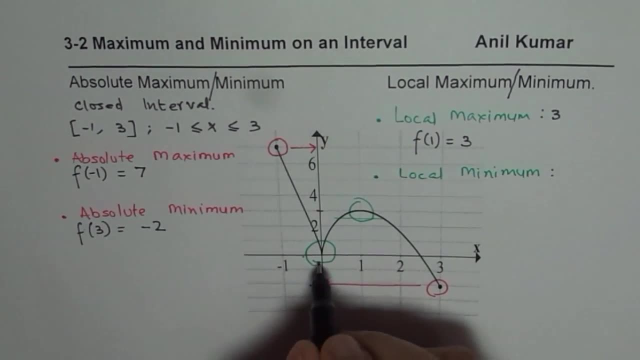 So f of one is equals to three, And so the local maximum is at one. So f of one is equal to three And the local minimum value is at three. And the local minimum value is right there, at the origin. It is zero: f of zero as equals to zero. 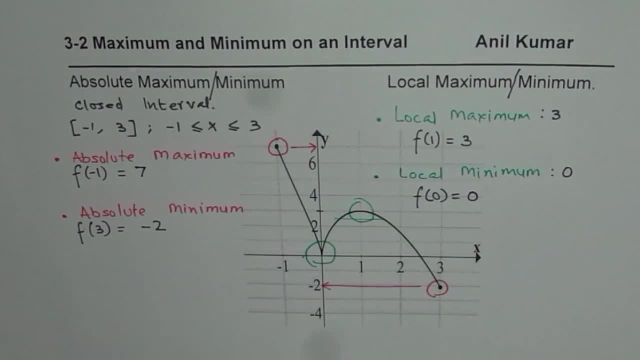 So in this chapter you are going to understand what absolute maximum is and what absolute minimum is, And you need to also understand what are local maximum and local minimum right? So absolute value means there is no other value in the given, only 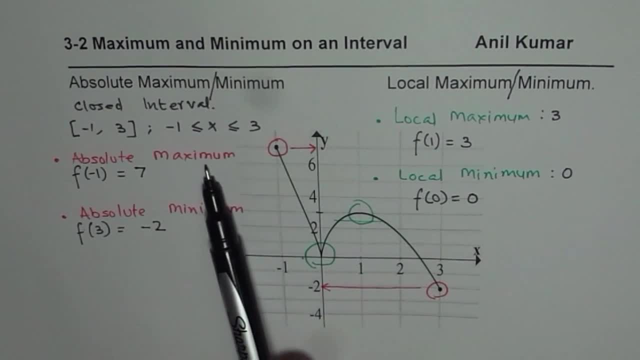 Which is participle or avelmentei, manufacturing with form In this case. other one is a little lower than الب MERS аilläهmen, That you can't tell is nor exist, but obviously you is more than that. then that becomes the maximum value, or less than that, it becomes the minimum. 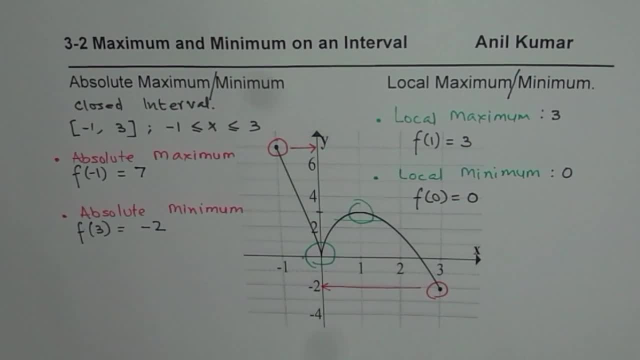 value right, and as far as the local maximum minimum are concerned, we look into close vicinity, so in nearby there are no other values which are greater than or less than that value right. so you get maximum or minimum now in terms of derivatives. what you will find is in terms of derivatives. 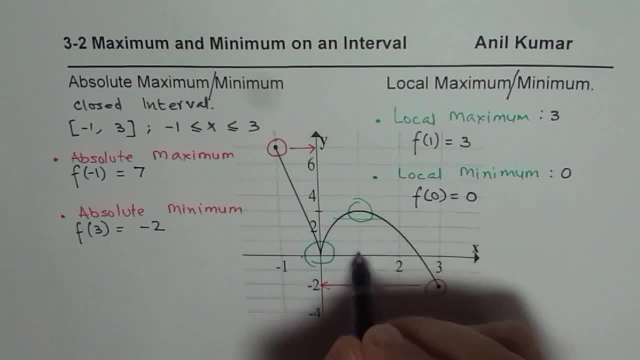 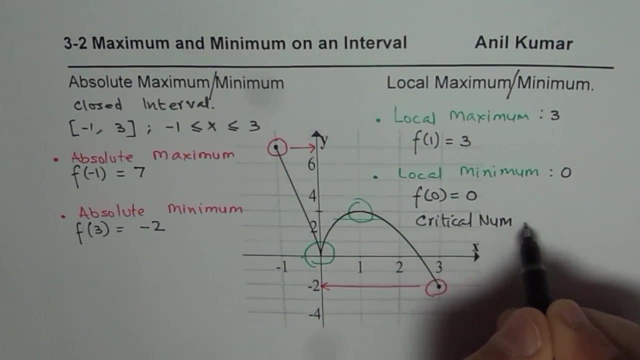 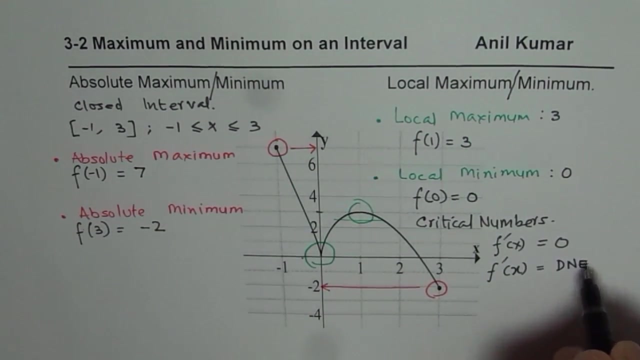 here. these are the turning points, so we call also them critical points. let me use the term critical points or critical numbers. so critical numbers are the points where the derivative, let's say f dash x, equals to zero, or the derivative f dash x does not exist. okay, or the derivative does not. 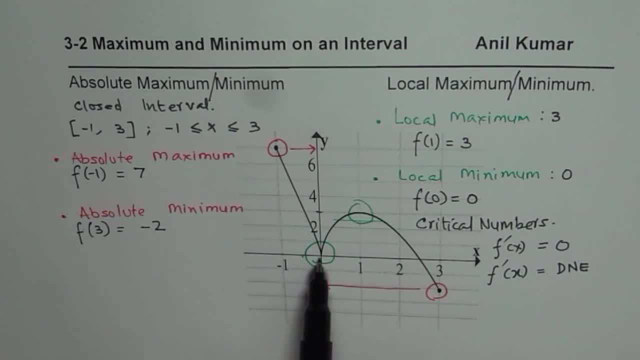 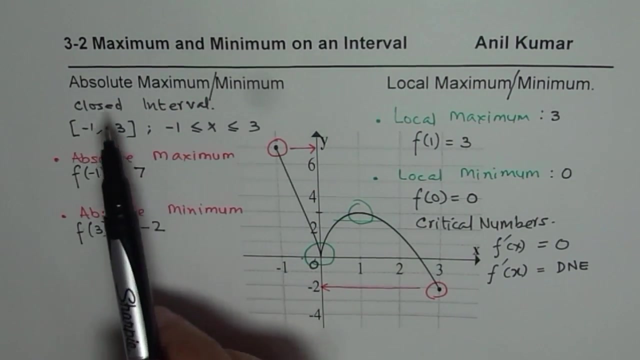 exist. you can see a cusp here. at this point, at the origin, the derivative does not exist and at that point we have a derivative which is zero, a horizontal tangent. so at such points we will get local maximum or minimum value. okay, now, whenever we talk about absolute maximum minimum, we have to.